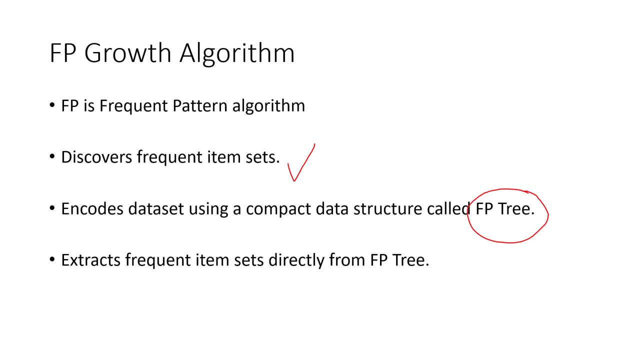 frequent item set directly from the f3 tree. very basic thing here we will do is we will consider the transaction table. from that transaction table we will extract the fp tree. from this fp tree we will extract frequent item sets. so we'll be using frequent item set for discovering association. 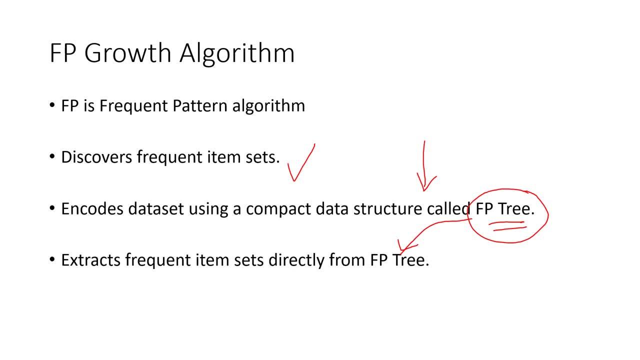 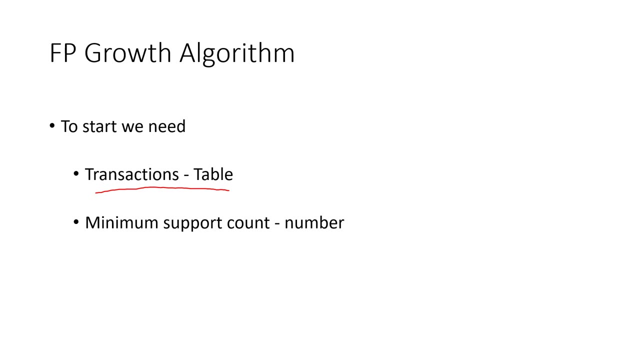 rules. so discovering the association rule is outside the context of this video. we will. i will only be discussing till how to extract frequent item set from fp tree. so, very first thing, to start with we need a transaction table and the second thing we need is a minimum support count. it is a number, so i will explain. 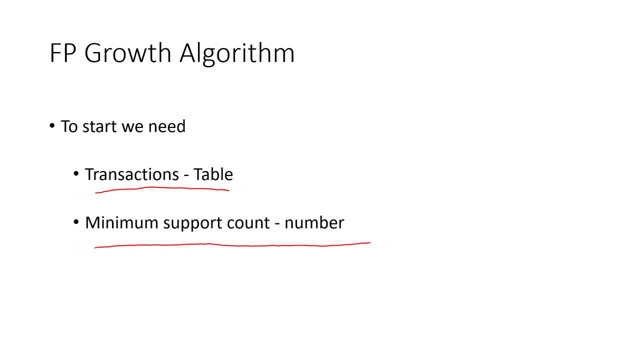 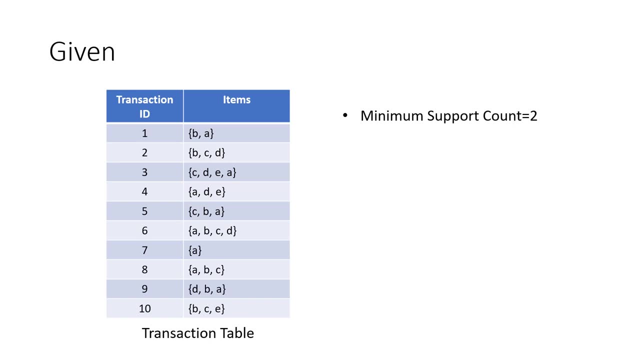 what is transaction table and minimum support quantity slides? so to begin with, to construct a fp train, to extract a frequent item set from fp3, you should be given two things. one is the transaction table and the minimum support count. so for those of you who does not know, 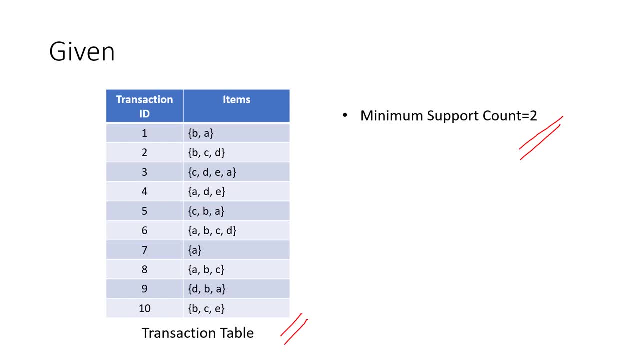 what is transaction table? transaction table is a set of items. it is a set of set of items, so wherein each set represents different items bought together. suppose you say in market or in a shopping basket. so b and a have been bought together, bcd have been bought together. 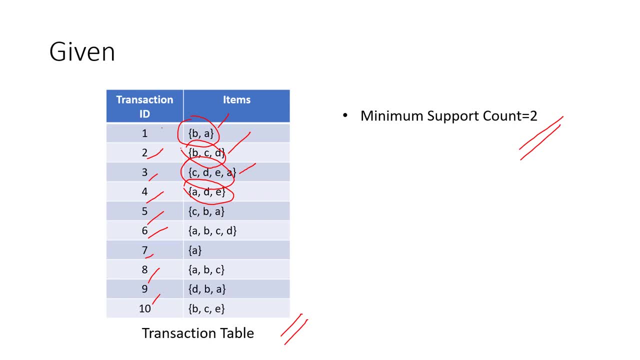 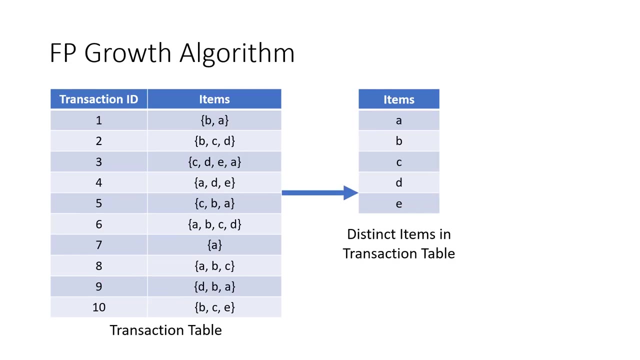 and we, our task is to extract the frequent item set from all this and the minimum support count. it is for any item which is having a support greater than or equal to two, then we will consider it as a frequent item. so, the very first thing, this is the step one, step one of fp growth algorithm. 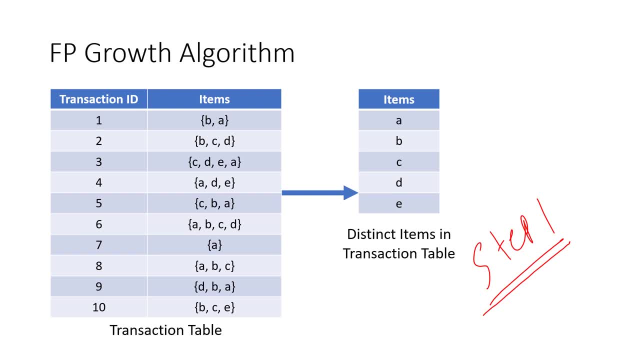 from the previous uh slide. we have taken this transaction table from the transaction table. what have done is from each and every transaction we have extracted the distinct elements. so if you can see, A, B, C, D, E are only the distinct element out of all these transactions. so this distinct item set we have for moving on. 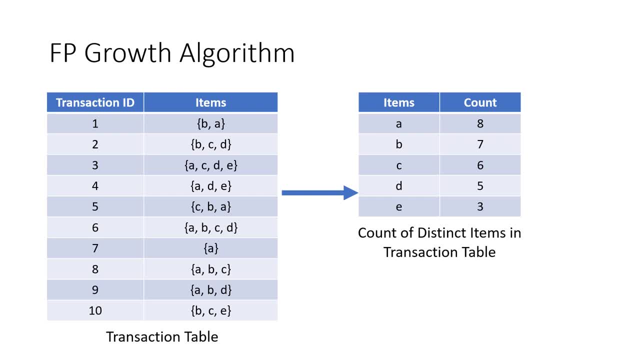 to the next slide. once we find out a, distinct items will count how many times each of these items have been seen in this transaction. the first item: if you want to consider a, he has been seen eight times. we shall let us verify a once twice. it tries fourth, fifth, sixth, seventh. so that is what the value of a is. 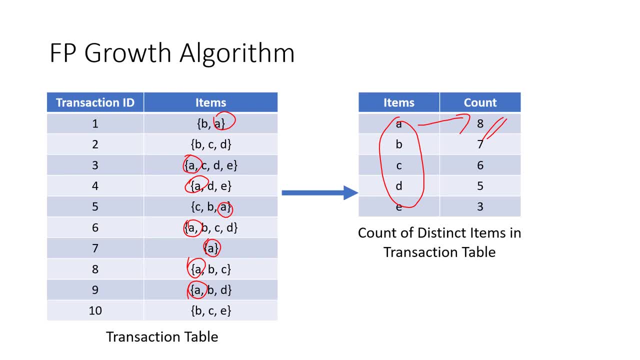 it, otherwise it could be more before. he has been seen many times in the transaction, so likewise we have only the total number of times to be seen in this transaction. is the total value of number of times we can see in this transaction? say, e and y are only like four and those depending upon the number of times on the? 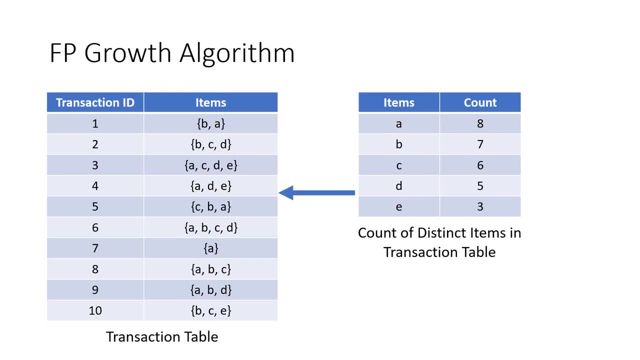 transactionwere to be reference example. we know that E has often a second place. B is the second payment and that means again the total contact that is fixed so day that the result will be P in the longer name. if you ran on the transaction table and E as a friend, then P and E are спокой absolutely. 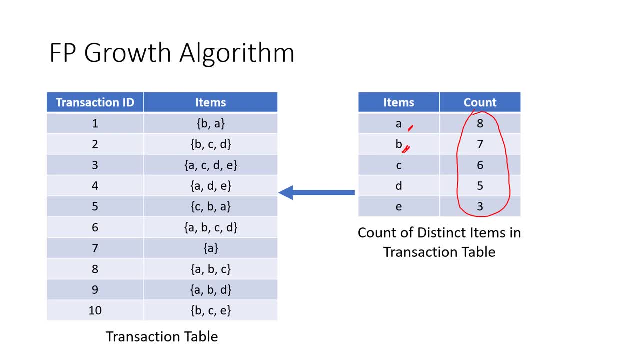 selected in the transaction table. two means we can also performing E. customers watch without fear can not be seen and the transaction table again takes maximum time and Mu is greater than b, for the transaction table has a intent following which also will break R T, which is see L times, p times B, which is dis errand of action table. 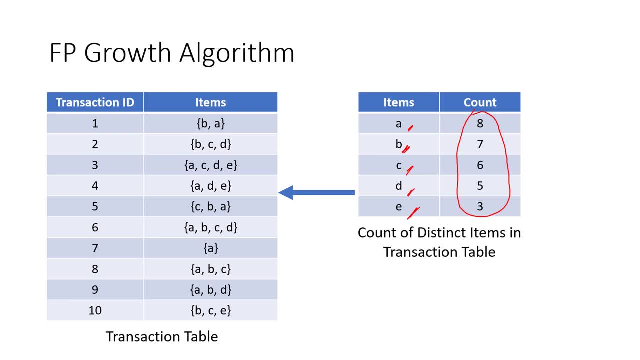 can be seen more number of times compared to d. d can be seen more number of times compared to e. depending on this chronology, you will have to rearrange the items of the transaction table. so here if i rearrange the items, so b is less in frequency compared to a, so we will rearrange the. 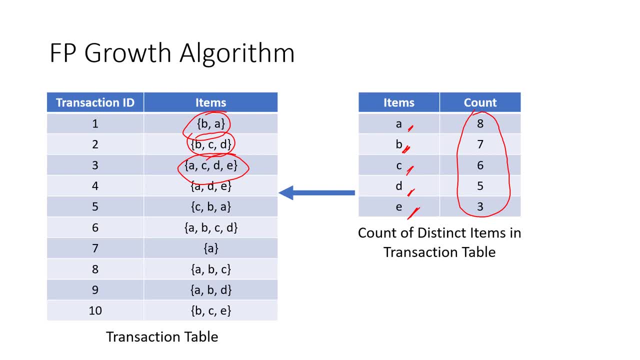 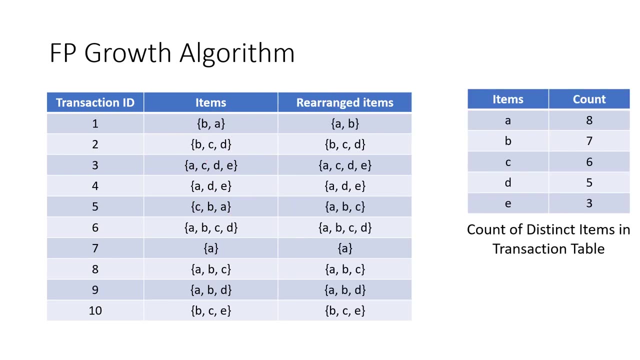 item as: a, b, b, c, d is in correct way. a, c, d, e is in, uh, correct way. b, a, d, e is also in correct way: c, b here. here you have to rearrange it: a, b, c. so once you rearrange, this is the original set of. 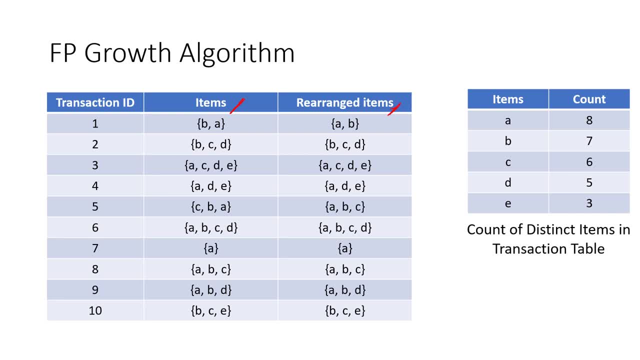 transactions. and this is the rearranged set of transaction. here you see, b has been rearranged to a, b and cva has been arranged to abc, and likewise the same thing will apply to every other transaction items in the transaction table. so let me brief once we have a transaction. 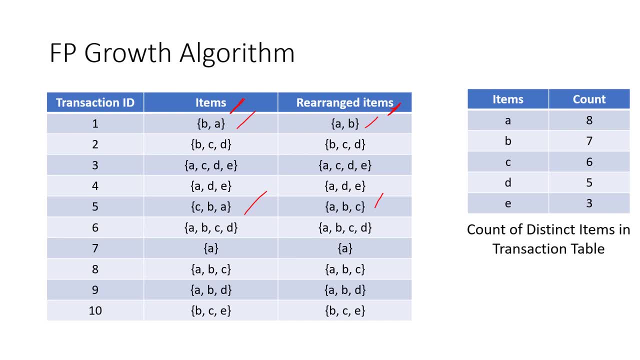 table and we have a support count. so far we have not used any support count. so, using the transaction table, what we had done was we had obtained the distinct items and we had obtained the distinct item count. so, according to: according to distinct item count, whichever is the item having the highest. 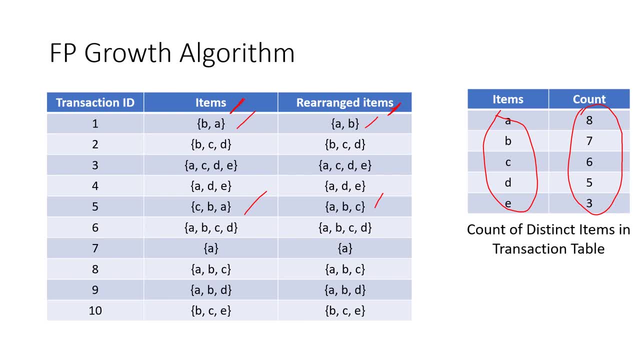 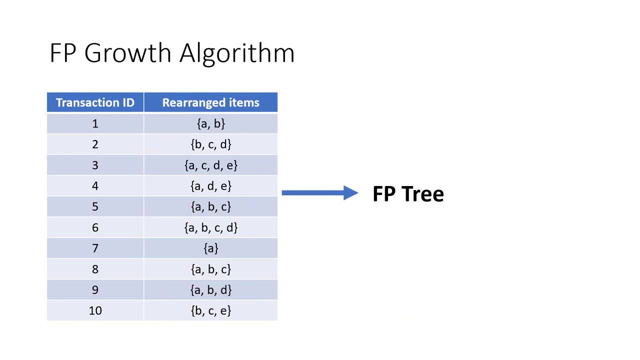 count will come at the beginning of the transaction set and likewise we have rearranged, so we henceforth we will be using this transaction table, which will not be using this transaction table, so, as i said, i will not be using this one will be using this one for constructing the application. so our basic 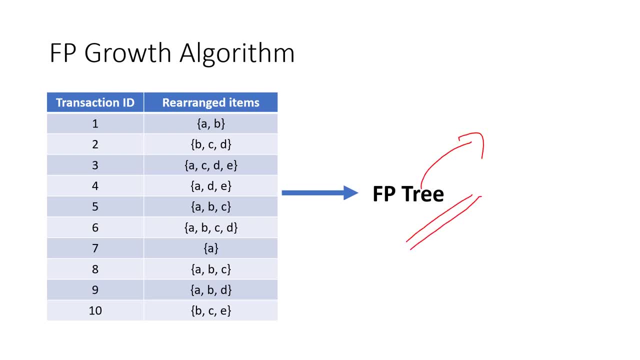 need is to construct that picture already. i have told we will extract frequent item sets from fp tree. so our goal is now to extract the fp tree from this transaction table. so to be more precise, it means we are using this fp tree on the foreign sectionanız. we are using the. 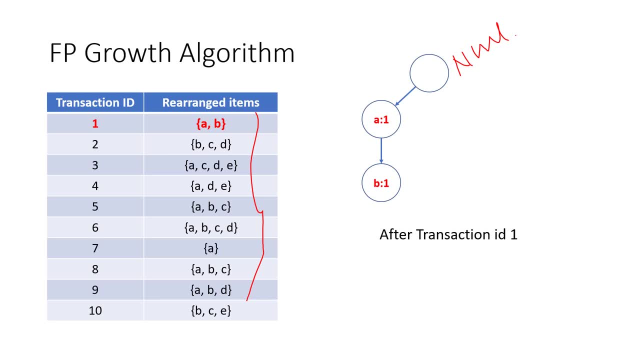 oral transaction column. we already have ganz and we still have some documents that are papers to spectrify after that process. so finally, for the very first company. so the topic we are going to deal with is that we only use a single common秒: war robins. 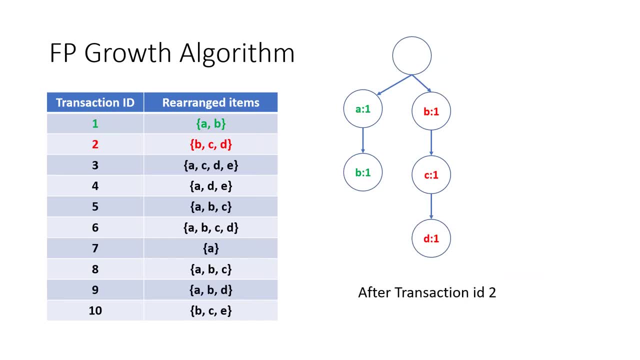 to use this as the binary, because if we exploit- and this is the first condition in our group, as i said, we have to use in a bunch of data and if we can do it, we will tomabe use the two잡ect rule first, but before that, with claim the first and second we need to. 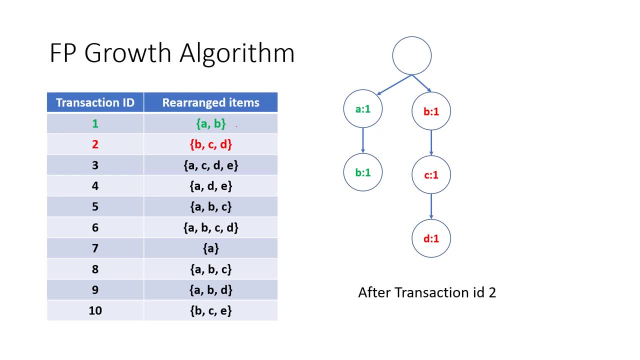 to use in as very in each other, in each of the random, and then we will use a convention: the transaction which we have scanned in green color and transaction we are scanning in the red color and all the unscanned transaction in the black color. so a and b in the previous slide we 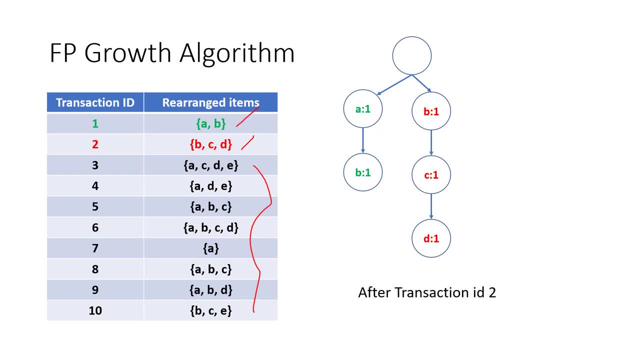 had seen we have already. it is a branch and the next transaction is bcd. so i cannot right away start with a b. b is not a node connected to the null root node, so i will start one more branch and assign the frequency of b occurring in this path: b1, c1. likewise b1, c1 and d1 in the second. 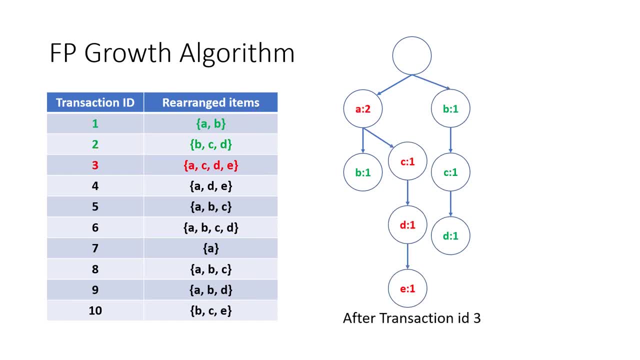 transaction. so likewise i will form one more transaction here. you can see, i am reusing the node a because the third transaction, acde, has been already seen in the first transaction. we had seen ab already. so that is why a and a, both are common here. so i will reuse this node to grow. 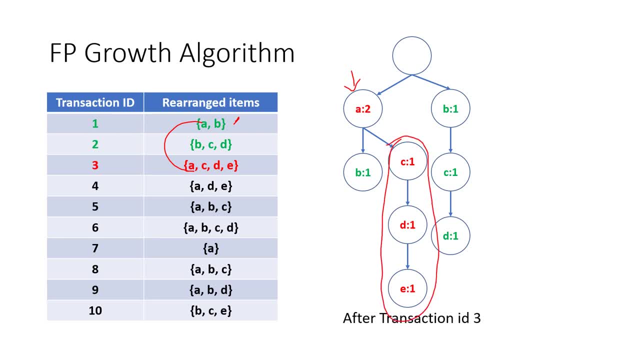 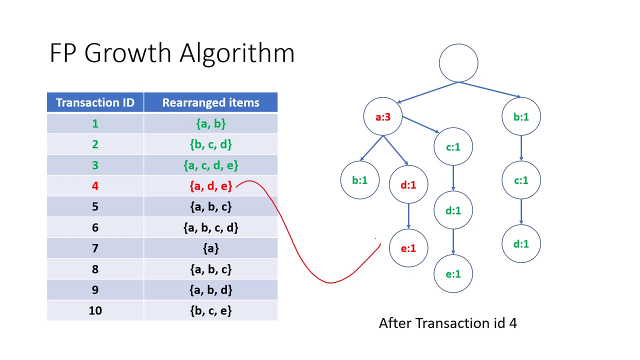 the tree from this point. so here the count of a becomes two and the remaining count will remain same. okay, cde, this is what we are leaving here. okay, likewise, we will scan ade, so a count becomes three and de counts becomes one one. so we will again scan: is abc, so abc, this. 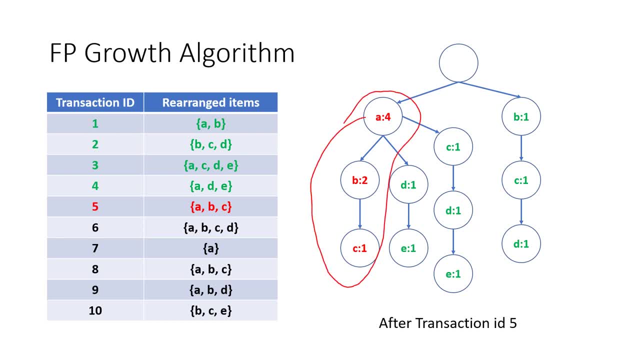 is the branch we will be okay, um. next up is scanning abcd, abcd. this is the branch we will grow. okay, the count of every element, whichever in the path, and getting in critical. you can see the. in the previous slide we had put a count as five, a count as four, sorry, um here. b count as two, but 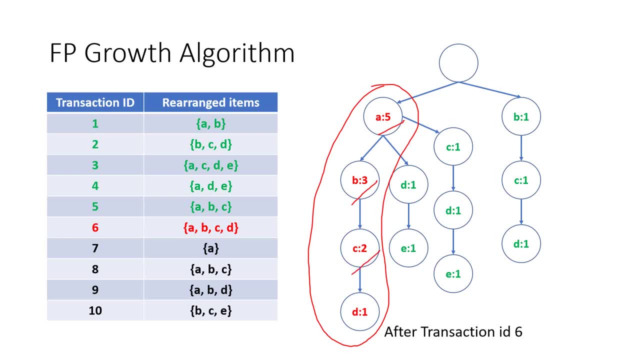 now we are increasing b equal to three and c count close one and the t count. we are increasing it to one because this is the new path. d count becomes one. likewise we will- this will relate to this- and a b c. this is the one we will see. this is a b c. we will scan the next item. this is the. 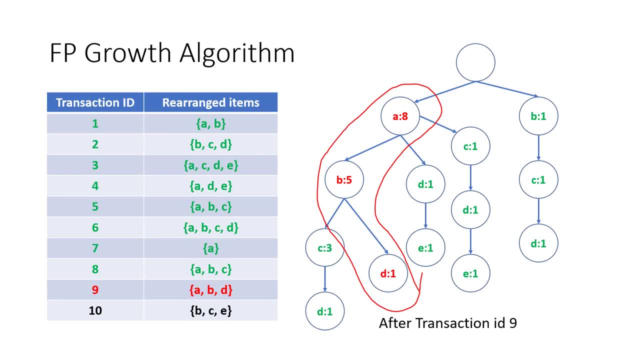 next item and the count of all the distinct elements in that path will be increased to pi 1. so one more thing: b c e. so this is the other part: b c e. so once we scan all the 10 transactions, this is the final fp3 we will be using for extracting the frequent item set. 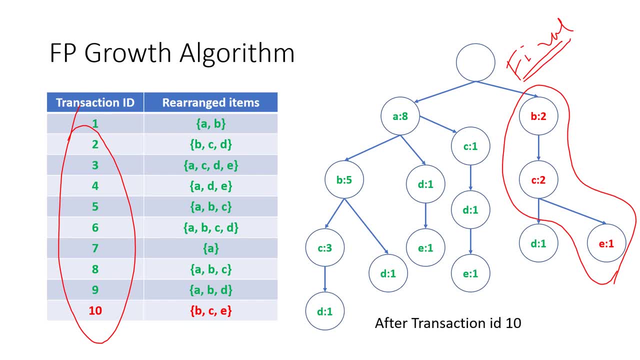 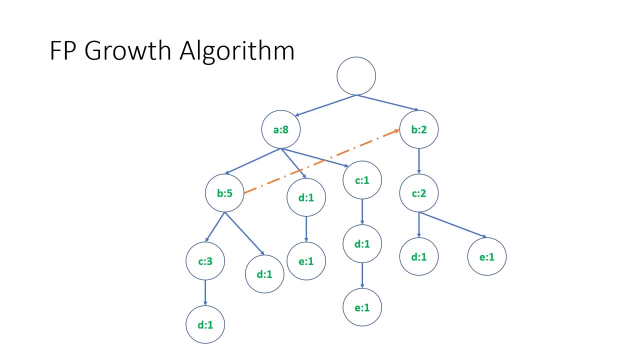 from the fp3. this is what we call it as fp3. so in some conventions there are some possibilities of extraction, the conditional fp3 in some cases. in some textbooks it has been given that they will add the dotted arrow marks between the corresponding elements, so you can choose to add. 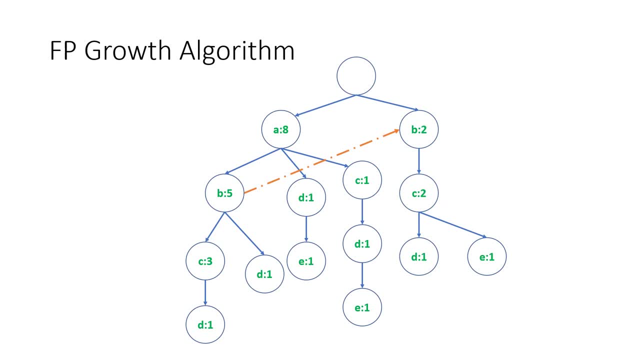 this dotted arrow marks between the corresponding elements. but it does not make much difference in the method which i am, we i'll be discussing here. so here, one more dotted arrow marks has been added in the corresponding here. so so the corresponding element c and one more dotted line has been added here you can see. 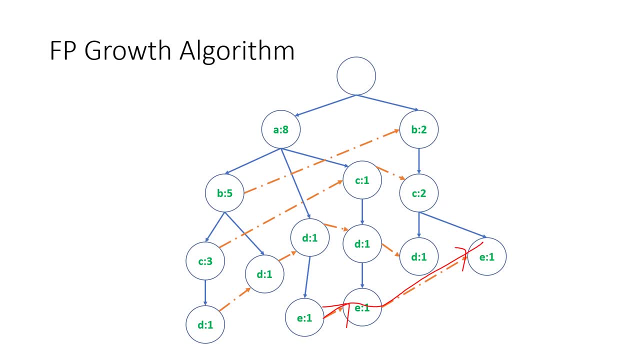 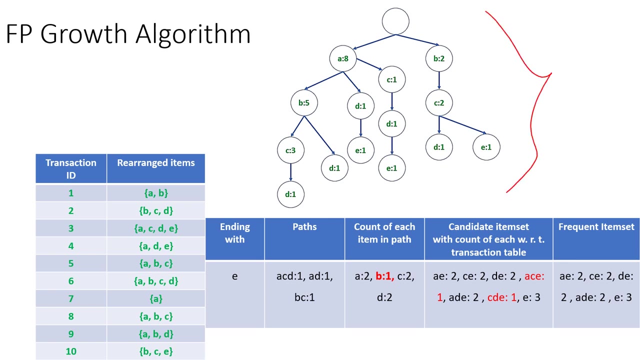 one more dotted line you can add here, so it is not not of much significance here for our discussions. so this is the final fp3, what we have. so once we obtain the fp3- this is the fp3 we have obtained from the previous discussions here- what we will do is we'll have to. 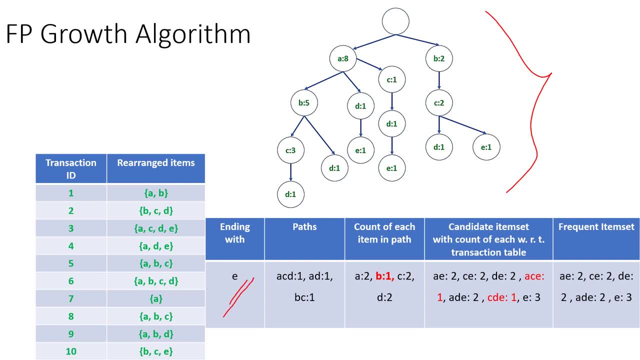 find out a frequent item set which are ending with e. to find out the frequent item sets which are ending with e, i'll have to consider the paths in the fp3 which are ending with e. so what are the paths which are ending with e? here is one path which is ending with e. here is another path which. 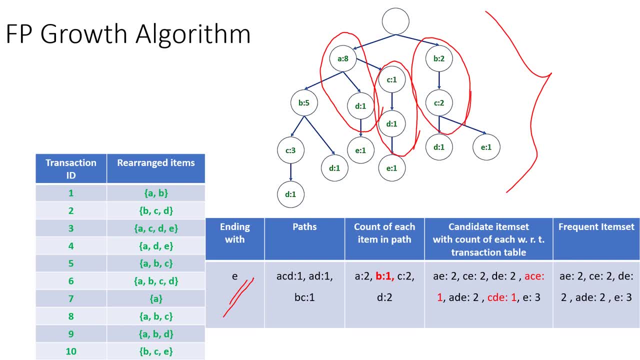 is ending with e and here is one more path which is ending with e. so all these three paths, um hello, all these paths will be written here. so a, c, d and the count will be one because e here is one and the count is one because the count of e is one. all of this count has been 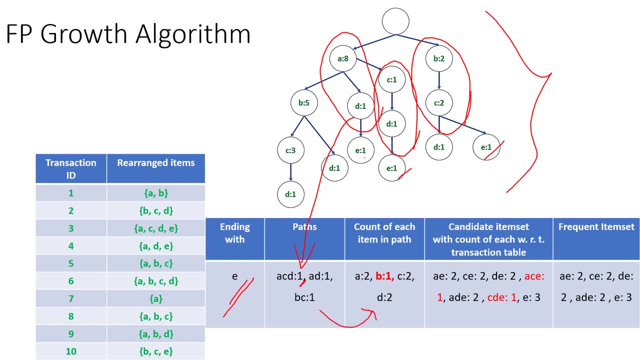 updated. so from this you will calculate the next column, that is the count of each item in path. so from this, how many times a has, from this, how many times you can see a, how many times you can see b, how many times you can see c, how many times you can see d. so from this we can infer: 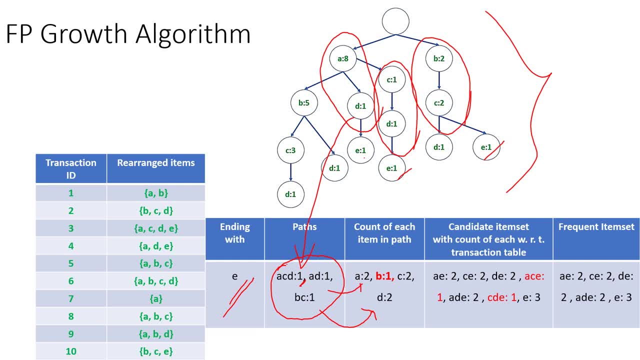 a can be seen from this two times, that is, in a, c, d and a. d and b can be seen only one time, if b has been, since only in this. b, c, c can be seen two times, so d can be seen two times. likewise, we have obtained count. 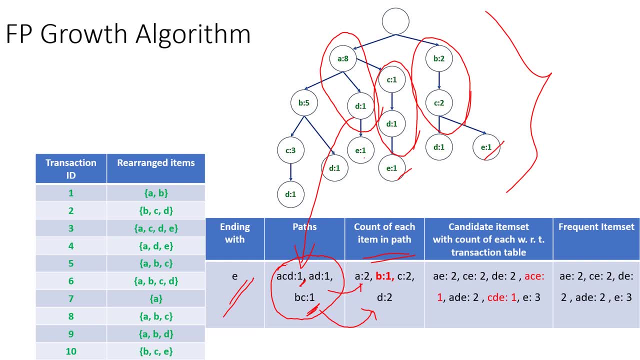 of each item in the path. once we count number of items in the path, as in the beginning slide we have, the support count is equal to 2. so this is what we had already discussed, so that we will count here. so, before doing going to the support count, what we will do is we will try to form all the item sets, okay, all. 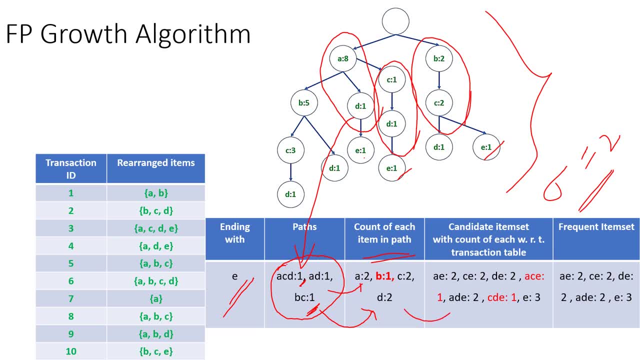 the item sets which are possible from this. so A is one possibility, because we are considering all the items ending with E. C is one possibility, D is one possibility, E itself is a possibility. A, C is also possibility, D is also possibility, C is also possibility. and all the combinations from whatever from. 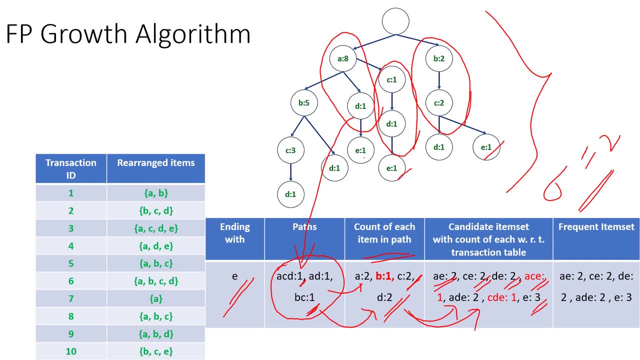 the this item set we have taken, we are writing it here, okay, okay, so we are not considering B. B is can be seen only once and our support count is 2, so from here again we will count how many times A, E, how many times A, E, C, E. 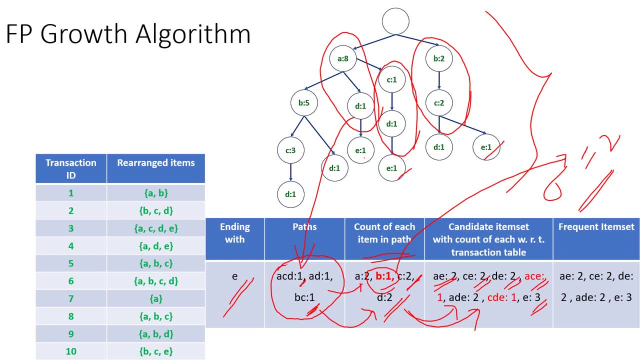 so here from this candidate item set with count of each with respect to transaction table, we will obtain the next one. whichever of the candidate item set having the support count, less than one will be eliminated. so they'll be promoted at frequent item sets. so here we have finished with E and C, how to find. 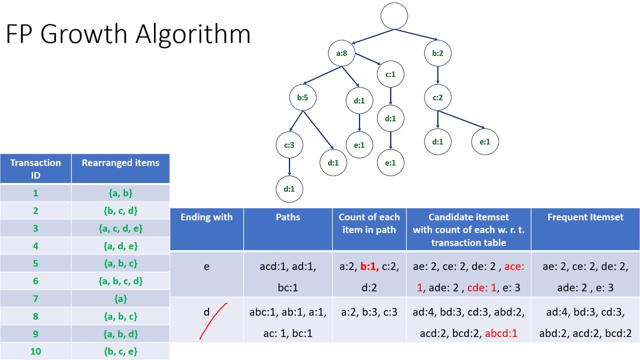 out the frequent item set using the path which are ending with D. so here the path. so we will identify. this is the path ending with d and this is also the path end with d. and here is one more path ending with d. and here is one more path ending with d. these are the all. 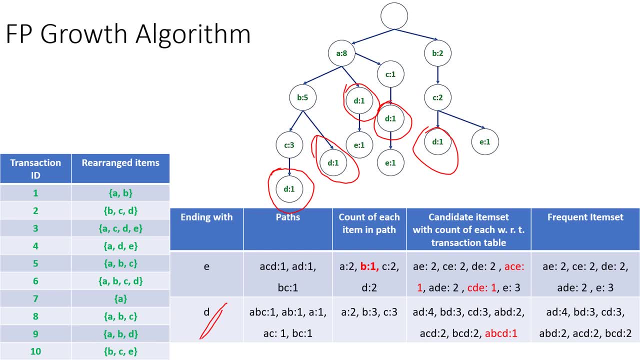 paths ending with d. so a, b, c, this one, okay, and a, b, this one, so a. here you notice, the count of a is given as one, because the d count is one, and here we have ac, and likewise from this we will count number of times each and every distinct element has been seen. 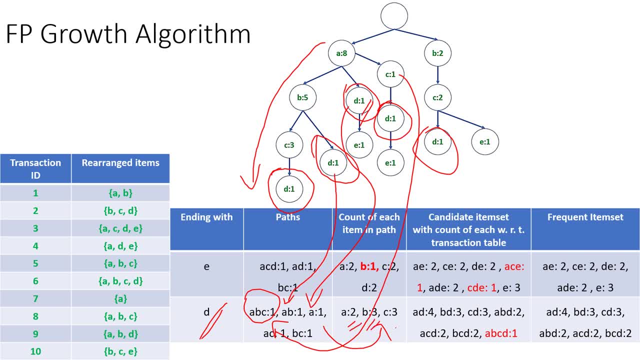 in the path: a becomes two, b becomes three, c becomes three. the count we had done from this distinct element, whichever are having the less support count- that means i meant to say which are less than two- will be eliminated. for our case, here we don't have any items which are less than two. next, the same thing will be used to form a candidate. 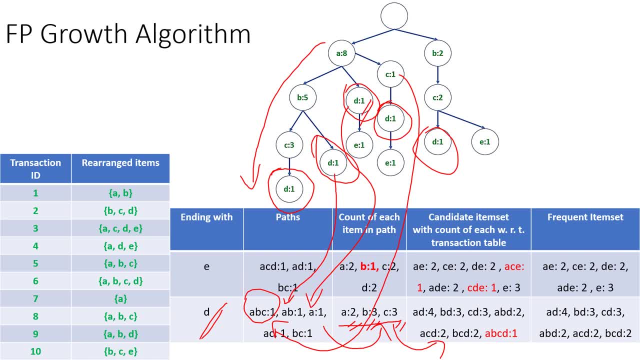 item set mixing with the d. so ad, bd, cd, abd and all the possible combinations have been listed here. so from this possible combinations we will count each and how many times ad has been seen, bd has been seen, cd has been seen and all other candidates have been seen in the transaction. 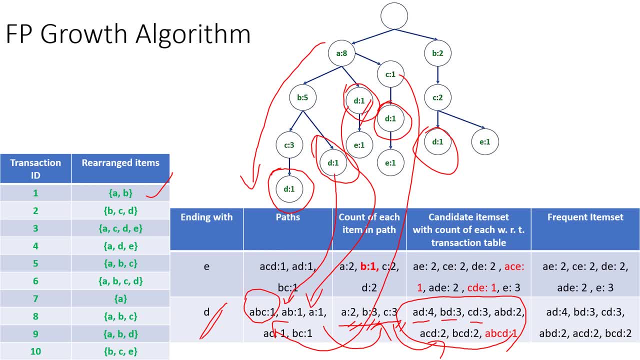 table. so ad we can see according to it, or we can see ad2 times, that is, one ad4 times. sorry, two, three, four times. so it is four times. so likewise we have counted all other elements. so whichever are the items are having the support count less than two. 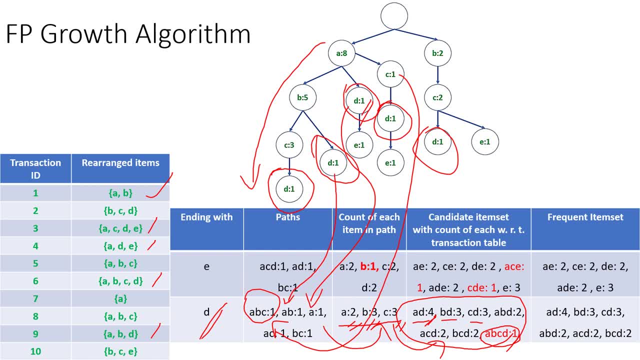 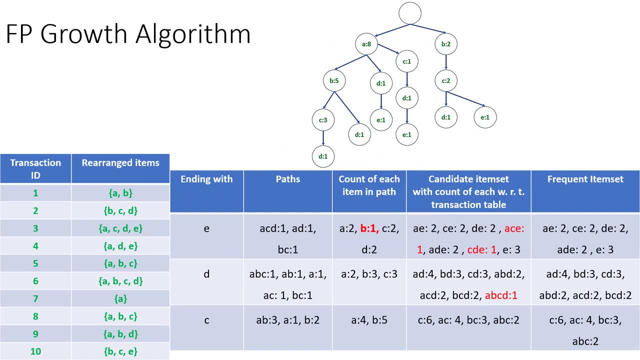 will not, will not be promoted as a frequent item sets, so this set will be return by eliminating abcd because the support count is less. so we will go to the next. the path sending with c. this is the path ending with c and this is the path ending with c. this is the 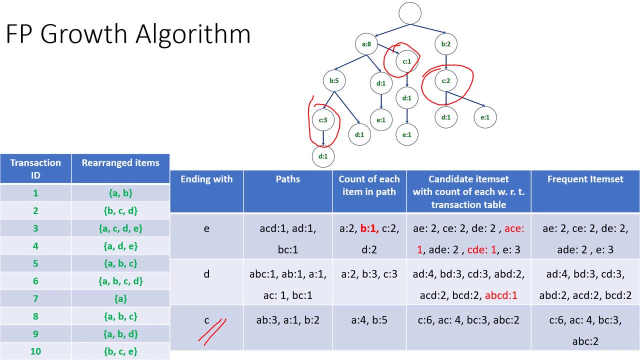 path ending with c. so here is the candidate item set which we follow on the previous process. from this we locked in this, from this will be locked on this, and this will be calculated in the transaction table. and any one of the items which are having the support count less than two, it will be. 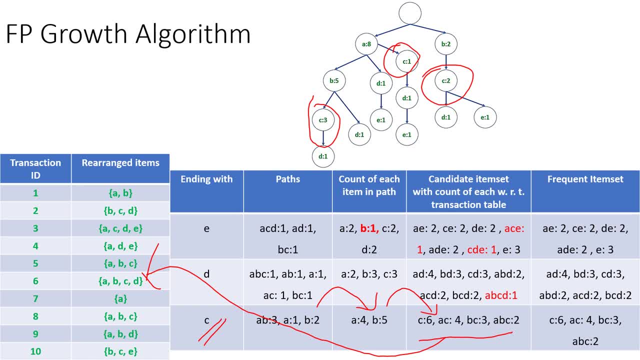 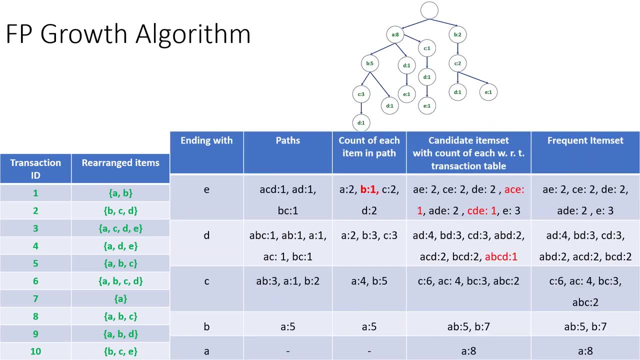 eliminated here. in this case we don't have any items which are having the support contrasting two, so we will promote it here. so likewise, we will repeat it for all the items b and a as well. so finally, we'll be having frequent item set. these are the frequent item sets. so here we have the 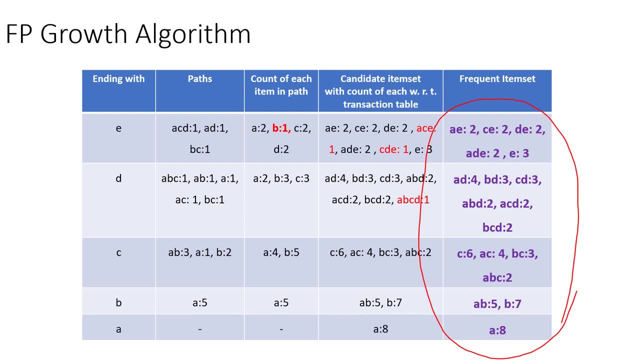 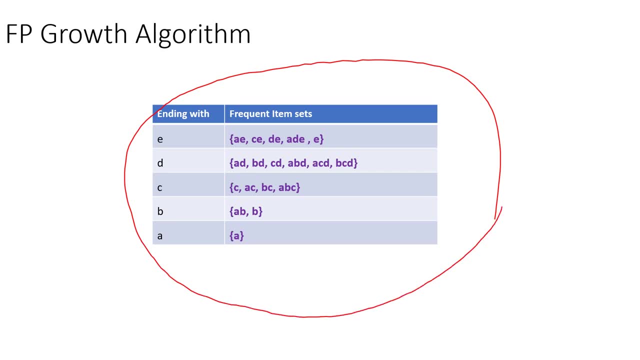 frequent item sets. so once we have this frequent item sets, we can use this for generating the association creation rules. so this is the first part for obtaining the frequent item set. obtaining the frequent item set is the basis for extracting the association rules. so in this video we will not be discussing